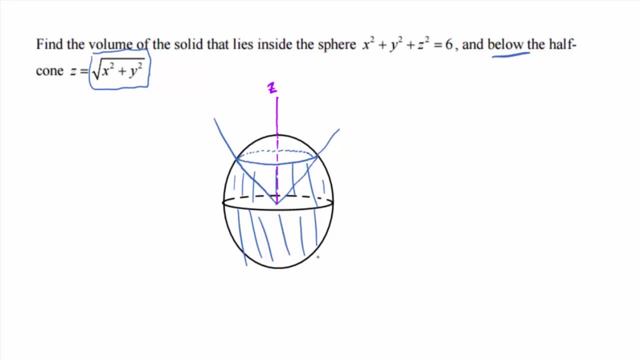 Okay, Okay, all the volume in the sphere kind of surrounding the cone, the bottom of the cone. does that make sense? okay, so let me erase those extra lines, because it really makes it look ugly. okay, so everybody's with me on what it is we're finding. okay, then, the only thing that's in question, if 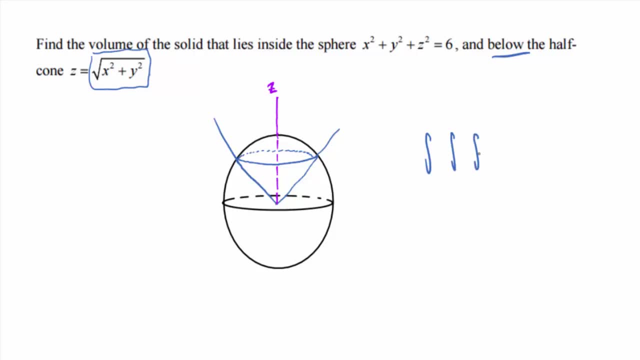 you think about it would be a single limit of integration that might be hard to find. the rest of it will be fairly routine. okay, so Rho squared sine Phi D Rho D Phi D theta. what does Rho have to run from? so this is going to be the volume, what there's gonna, we're gonna. 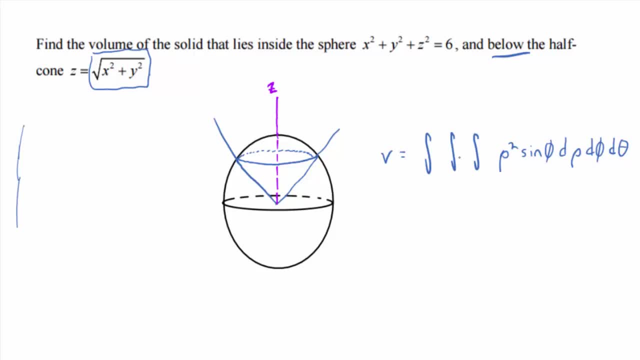 have to do some more work over here to get one of the limits of integration, but I want to point out that you can just visually inspect it and get all the limits of integration except one. so what does Rho run from zero to root six. okay, now, this is. this is the one I was talking about. 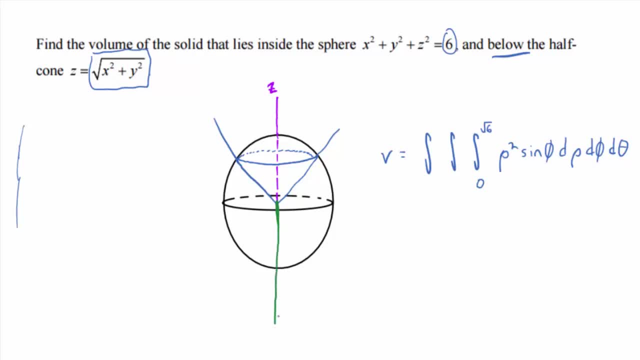 if you, if you think about it, here's the negative z-axis down here. if you think about what Phi has to range from, here's the initial side of Phi. right, we actually want to start Phi here, don't we? and then run it all the way down here. 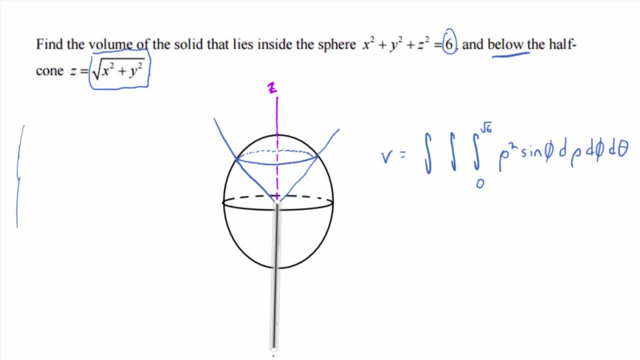 well, I know what this angle is down here. so I know, actually, the upper limit of integration, right. so the upper limit integration, integration on Phi has got to be Pi, right, but I don't know what. no, this angle is my Phi one, though I'll call Phi one the lower limit of integration. right the angle, the 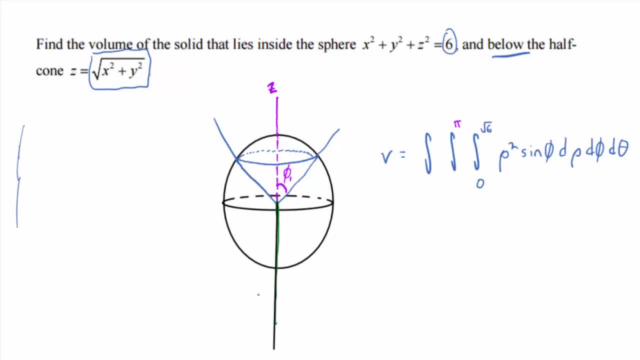 side of the cone forms with the z-axis. so that's my Phi one. that's what I don't know, right, I'm gonna erase that in a second, so don't write that down, but I'm gonna figure that out in a second. then what is theta gonna be? 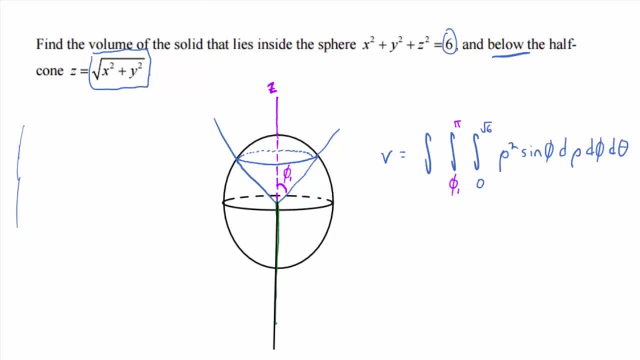 to run from. I mean, if you, if you project down into the XY plane, you're, you're gonna get that you're integrating over a disk, aren't you? well, I'm sorry, I made it too big. no, that's. that's actually fine the way it is, the way I drew it, think about. but you don't even need to do that when you're in. 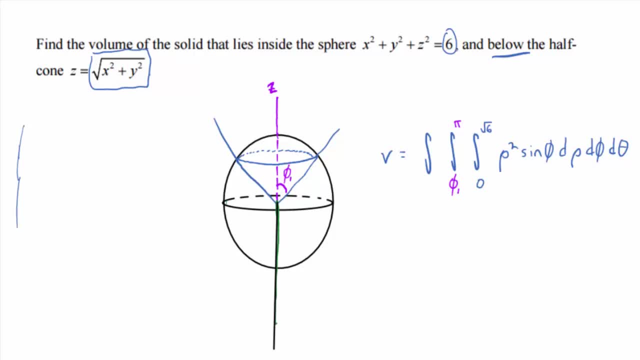 spherical coordinates anyway. so think about it in order to sweep out all the points that under inside the sphere and underneath that cone isn't theta gonna have to be at its limits zero to two pi. yeah, so do you see that just by drawing the picture we automatically know all the limits? 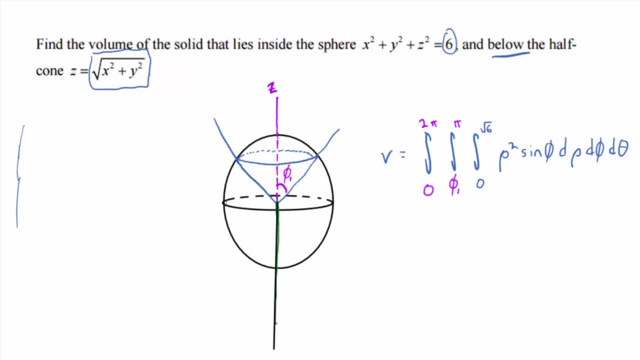 of integration, except the lower middle one. now, because it's z equals square root of x squared plus y squared, I can predict that it's gonna be pi force. but you had got to be careful because you know, on the test I might change it so that it's not pi force anymore. 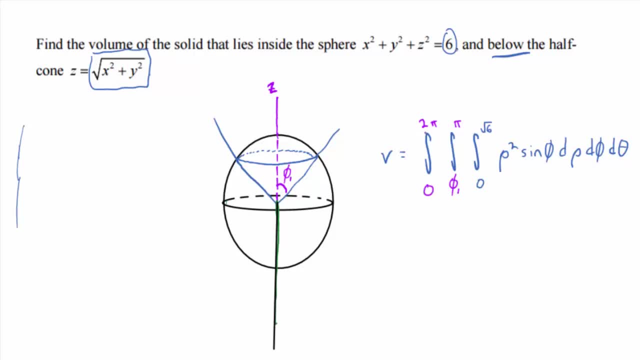 so let me show you kind of the generic way of finding that angle. then we'll go ahead. sorry, I've gone a little late. we'll go ahead and take that break. so well, no, I mean alright, so think about it. this would be a circle. this intersection curve would be a circle, right, okay? and then I 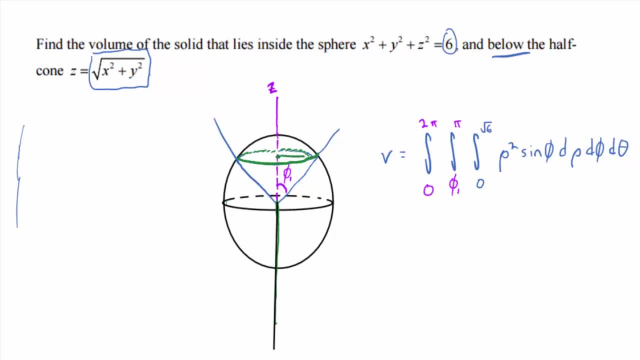 think, okay, could get the radius of that circle fairly easily and then I could focus on this triangle to help. it's a right triangle and I could focus on that right triangle, including the radius of that intersection circle, and I could get fee using just right triangle trig if I can get the radius of that inner of that. 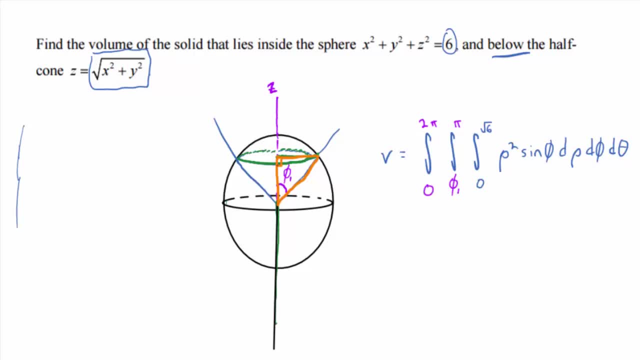 inner section circle, so the intersection circle- in green they are the points of that circle- have to satisfy both. this fear in the colony. treat this fear in the colony equation like it's a system of equations and sacrifice equal square of Xbox y squared in there in square, and if I do that I would get. 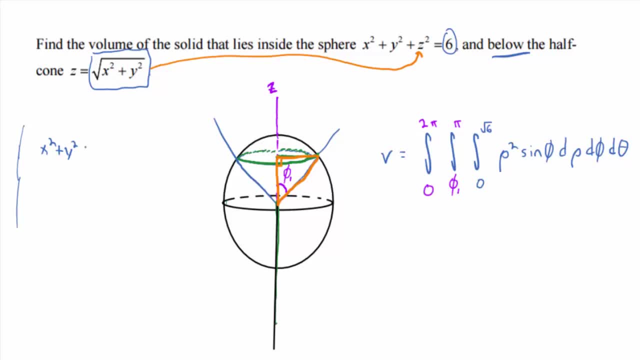 x squared plus y squared plus. while you square square, you get another square squared plus y squared equals 6, or 2x squared plus 2y squared equals 6, or x squared plus y squared equals 3.. Does everybody buy that? So what's the radius? 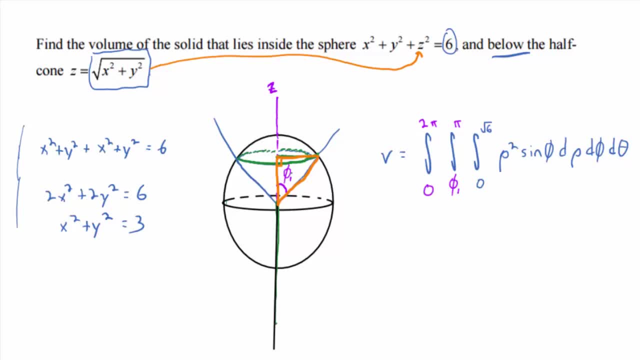 of this intersection circle in green here. Wouldn't it be the square root of that number? So the side of that. so I'm going to redraw that triangle in orange there separately so you can see it. So here's phi 1, and I know that the length